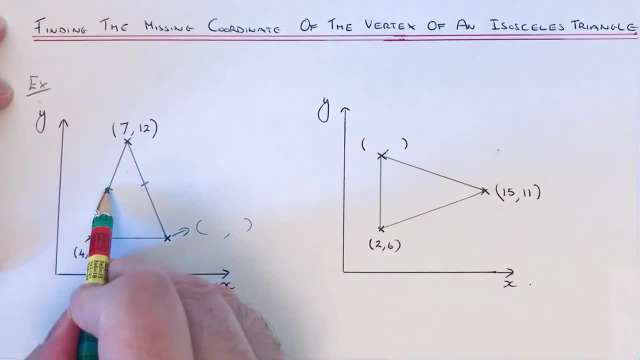 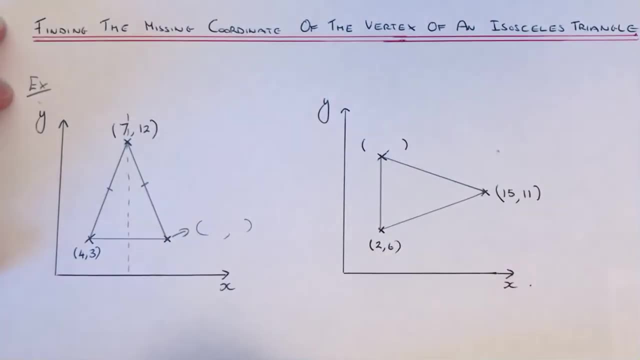 So we've got an isosceles triangle, so that means these two sides are the same and we have a line of symmetry down the center of the isosceles triangle. So the first thing you need to do on these types of problems is mark the numbers. 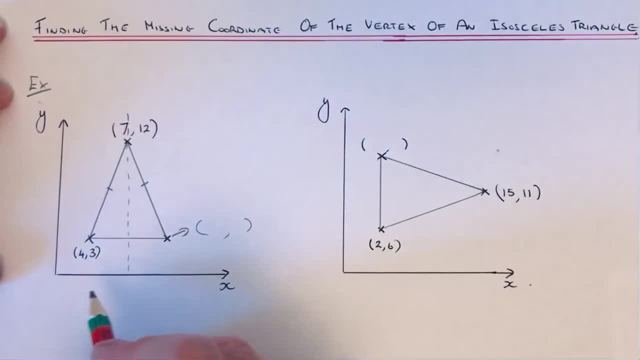 along the x-axis and the y-axis. Okay, so let's start with this point here. So the first number of our coordinate will go on the x-axis and the second, number, 3, will go on the y-axis. So do the same for this coordinate here. 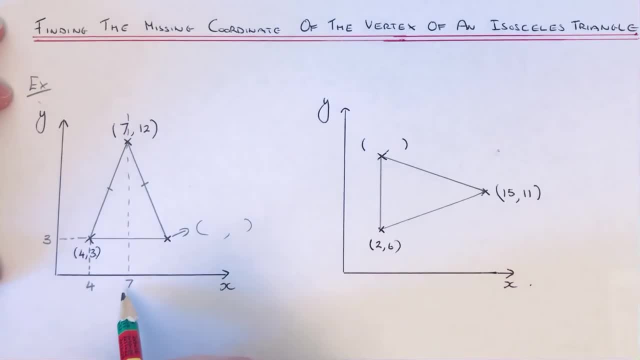 So the first number, 7, will go on the x-axis and the second number, 12, will go on the y-axis. So we now need to just find out what this coordinate is here. So we don't have this number along the x-axis, but we do have the y-axis number. 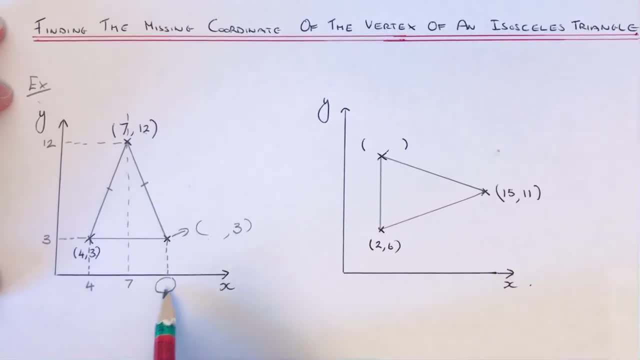 which is 3, so we can fill the 3 in there. So we're, just after that, first x coordinate. So to do it, we can look at the numbers along the x-axis. So if you look at the difference between 4 and 7, it's 3, isn't it? 7? take away 4 is 3.. So if we add 3, 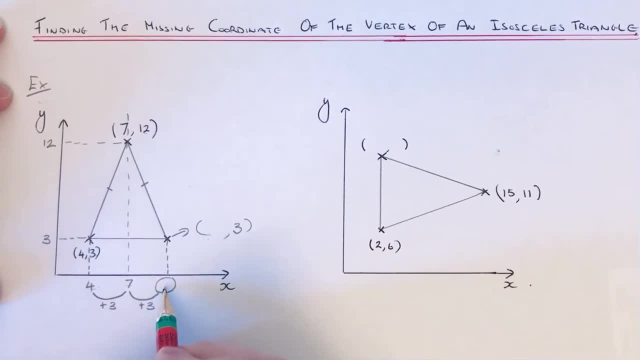 on to the 7 that will give us this coordinate here. So 7 and 3 is 10.. So the x coordinate is 10.. So let's have a look at the second coordinate. So we're going to look at the second example then. So again, we've got another. 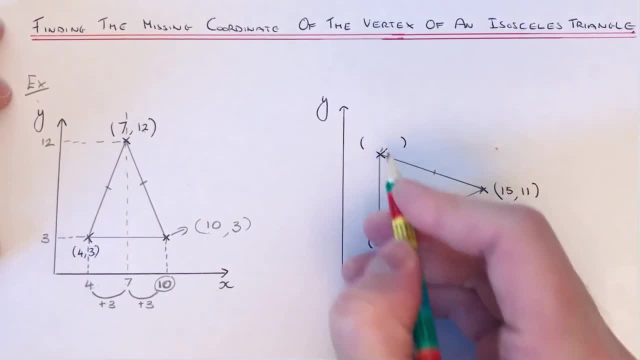 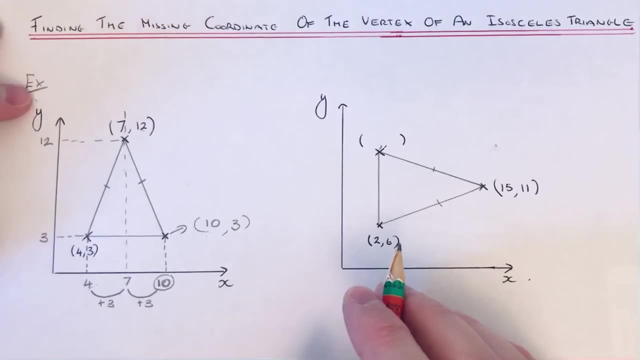 isosceles triangle and we need to work out the coordinate of the top vertex. So again, if we use the coordinates, we have to mark the numbers on the x and y-axis. So let's start with this bottom coordinate here. So the first digit will go on the x-axis. 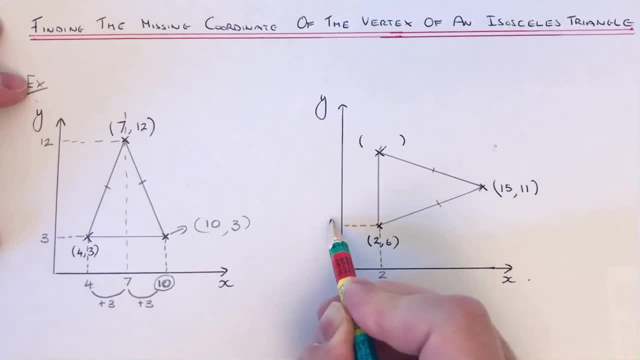 which is 2, and the second digit will go on the y-axis, which is 6.. Do the same with this vertex. so if you put the 15 on the x-axis and the 11 on the y-axis, and then we can just figure out.